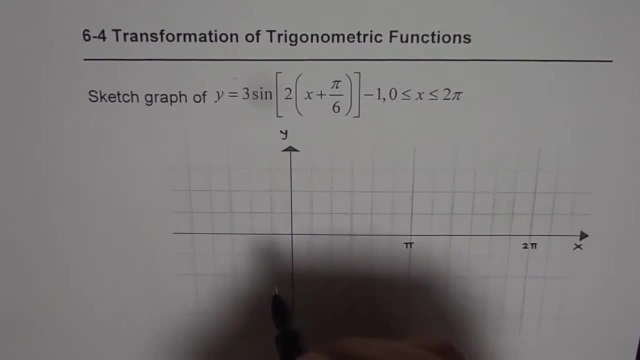 So this is the primary trigonometric ratio sine of x, and then see how it could be transformed. So what we're doing here is we're using each point as 1, and this will be minus 1 for us. I'm sketching it in very light colour so that we can highlight the transformed trigonometric. 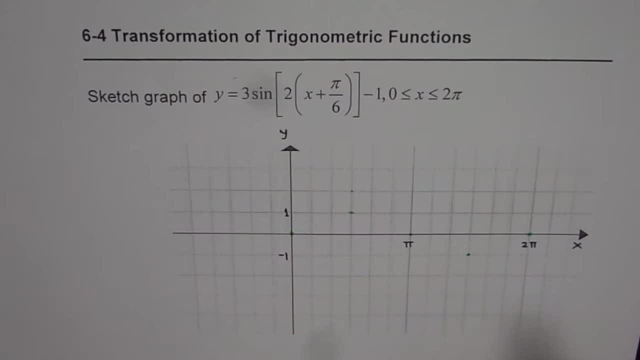 function with a darker color right. So sine x function normally will look like this. So that's one wave of sine x which has maximum at pi by 2, minimum value of minus 1 at 3 pi by 2, right, And zeros at 0 pi and 2 pi. That also gives us the key values of sine function to work. 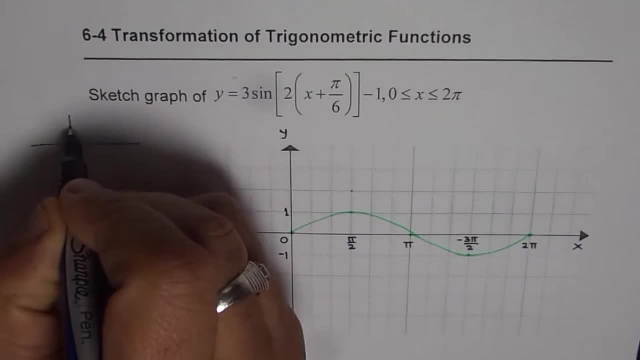 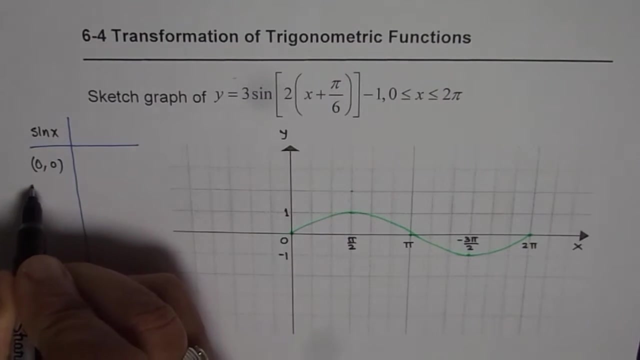 with right. So here I'll make a table giving key values for sine of x right. So we'll start with sine of x. Key values for sine of x, as you see here, are: 0,. 0, starts with origin, pi by 2,. 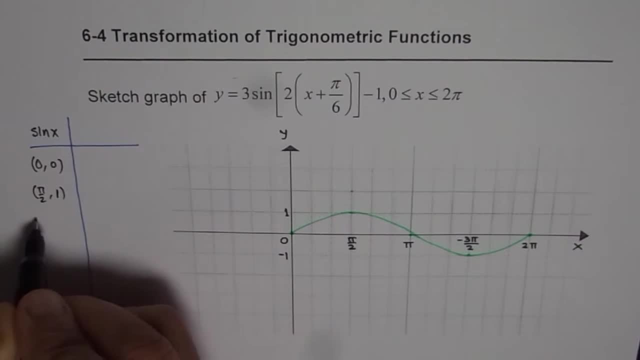 plus 1, that's the maximum. Then we have next 0 at pi and minimum at 3 pi by 2 and then 0 at 2 pi. So these are five critical points on the function sine of x. If we consider these five, 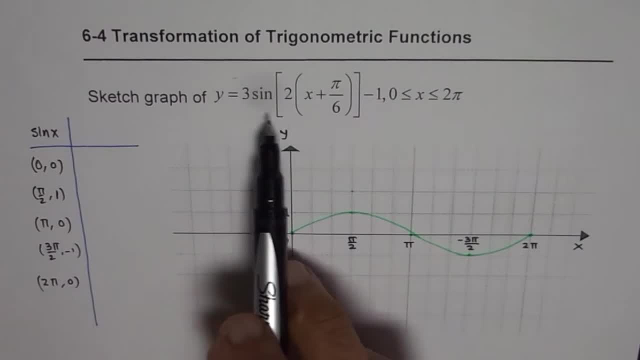 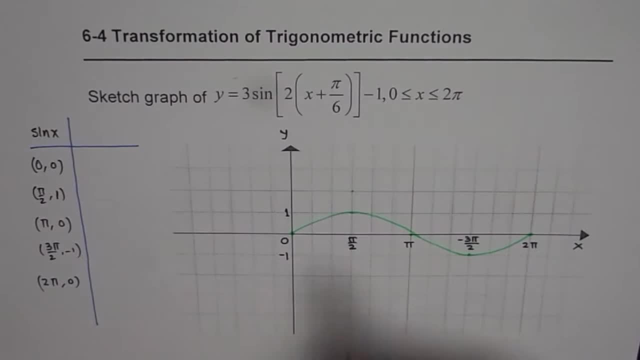 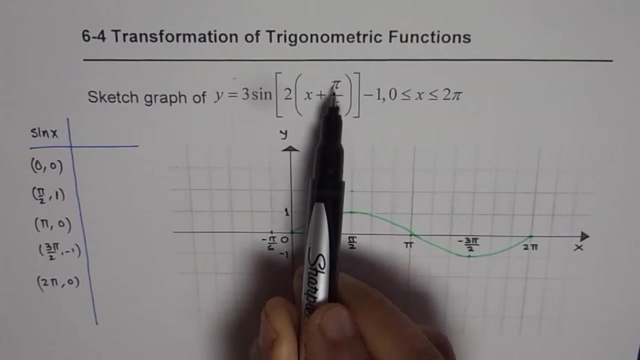 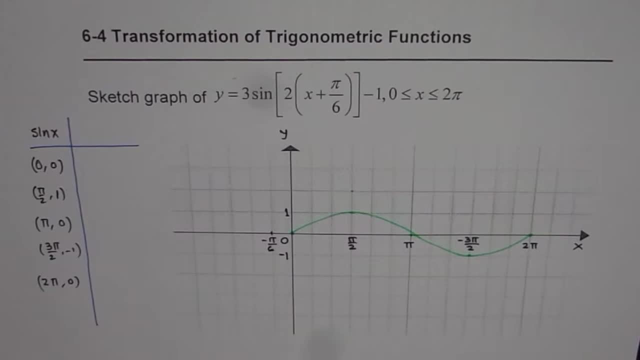 itself. so when we analyze the equation, what do we get? vertical is stretched by 3, that means amplitude becomes three times, and horizontally compressed by 2, it means in 2, pi will have two waves. right, that is what it means. k value of 2: 2 waves, that means time period will be pi for this particular function. 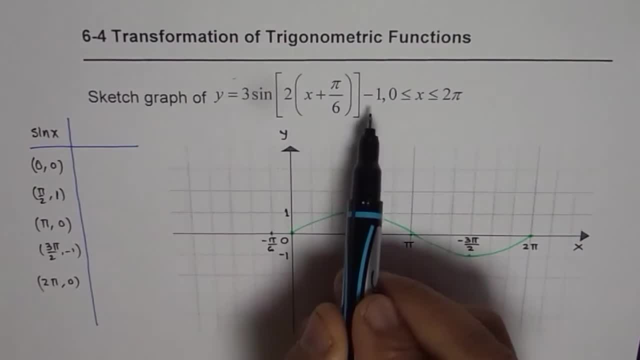 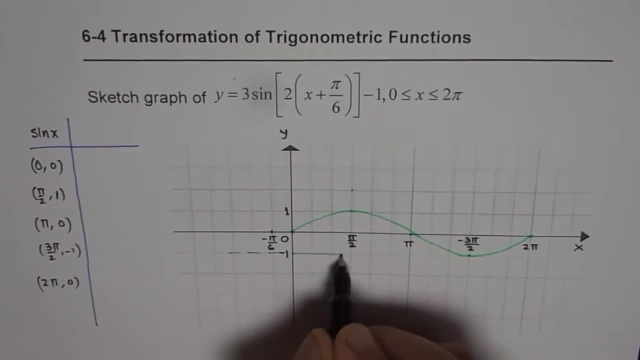 horizontally translated pi by 6 to the left, 1 unit down. so the Xs for our graph will be now here, right, so that becomes the Xs. let me draw in this light color correct, and maximum will be 3 more than this: 1, 2, 3. so that is our range. 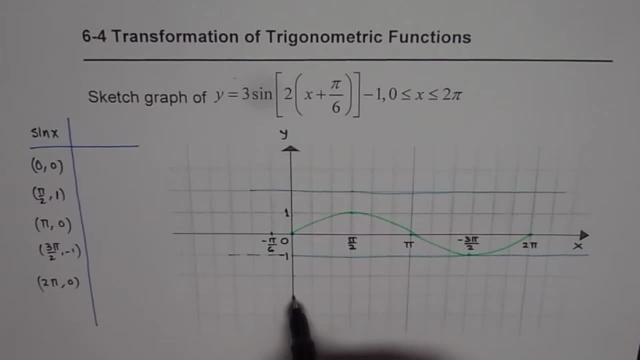 maximum side minimum will be 3 less less 1, 2, 3, minimally 3 less. So I'm roughly teaching you how to sketch it and this is very accurate method right Now here. time period when we say is half k is as you can. 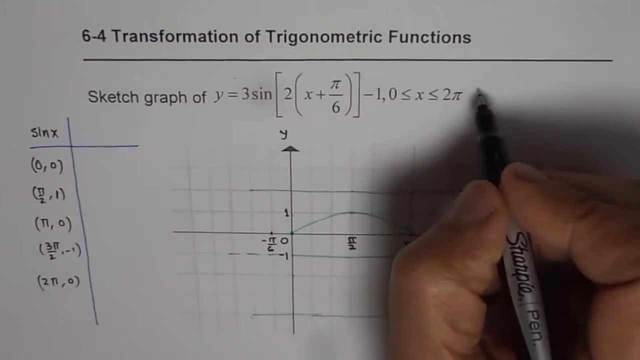 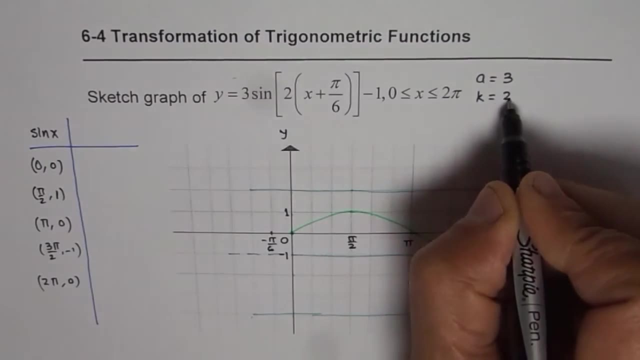 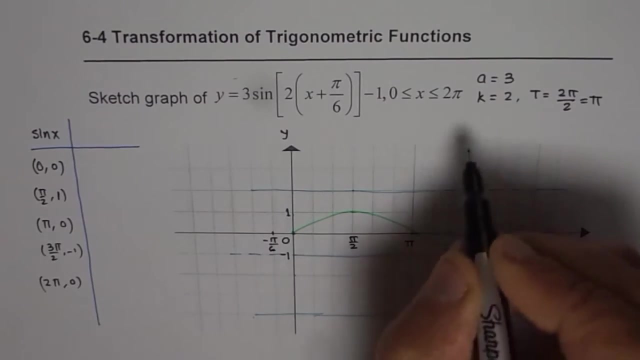 see here. let me write. let's analyze this. So what we have here is: amplitude is 3 for us right, k is 2, that means time period is 2, pi by 2, or equals to pi right And horizontal. 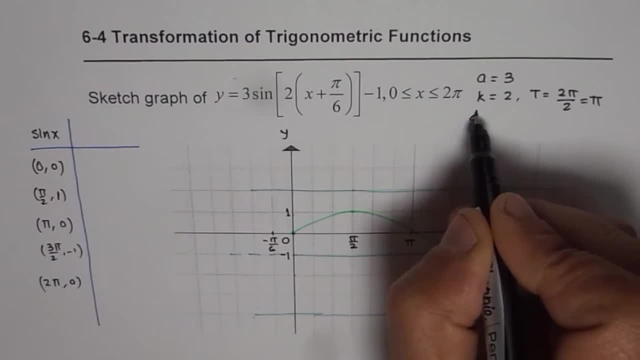 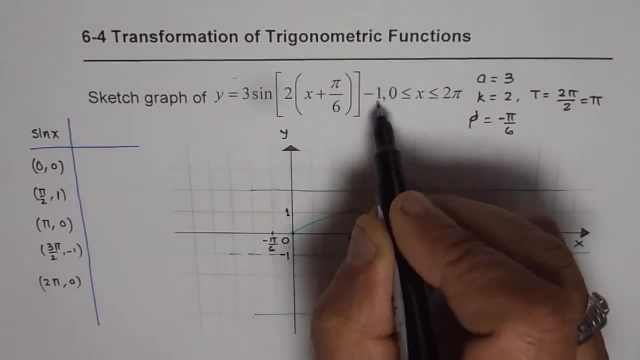 shift, which I can write as, let's say, p phase shift, p minus pi by 6, right, And moving up it is: let's say c is minus 1.. Xs, you can say right, Let me write xs. 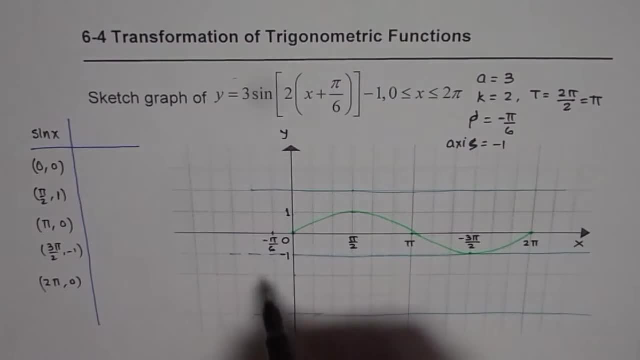 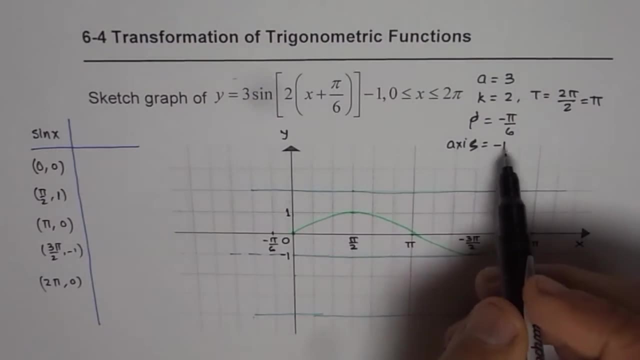 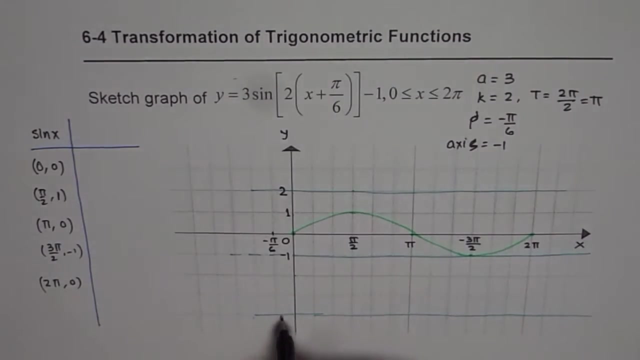 here, X is at minus 1.. So this is: X is at minus 1.. Amplitude of 3 will give me maximum value of minus 1 plus 3. That will be 2 and the minimum will be minus 1 minus 3, which is minus 4.. Do you? 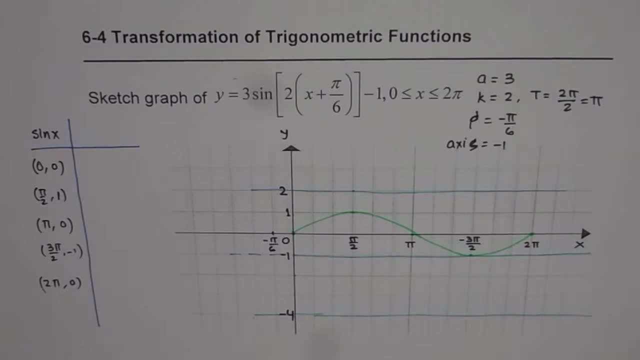 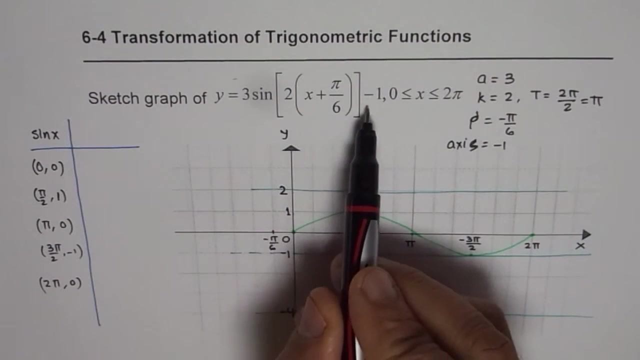 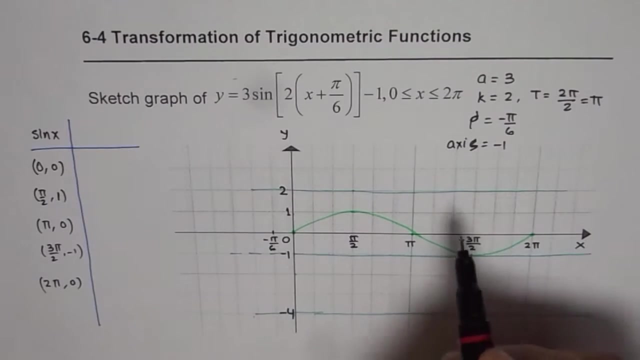 get the point right Now. what we can do now here is that we can perform horizontal stretch by 3.. Now let me first sketch without translation: horizontal right. We already incorporate vertical translation, Perfect, And we will do compression and stretch. So basically, 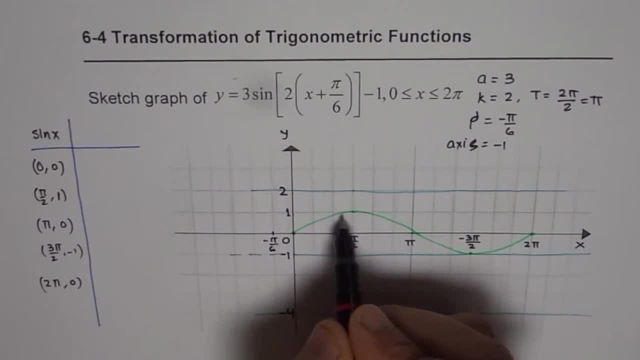 all these points will come half way, So this is at 1,, 2,, 3.. So it will be at 1.5 and stretch to maximum. So there it goes. This will be half way. So this will come at pi by 2.. 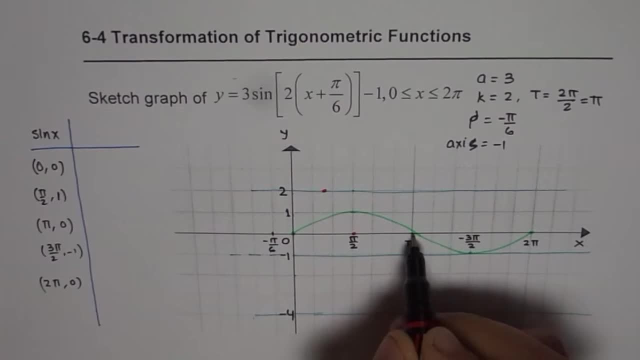 So we are stretching them vertically by a factor of 3 and compressing by half. So this will be: this is 6,, 7,, 8, 9 divisions. It will come at 4.. 1,, 2,, 3, 4 and a half right And vertically. 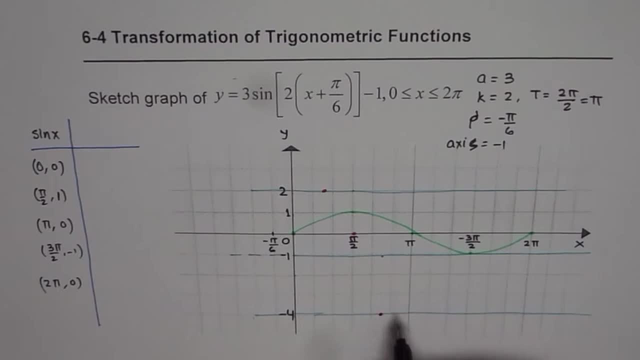 stretched by a factor of 3.. So it will be right there. So that is how it will be. Minus 2 pi. So it will be at pi on the axis. Do you see that? So 1 wave for us will be sorry, this point is here also moving 1 unit down. So we have done. 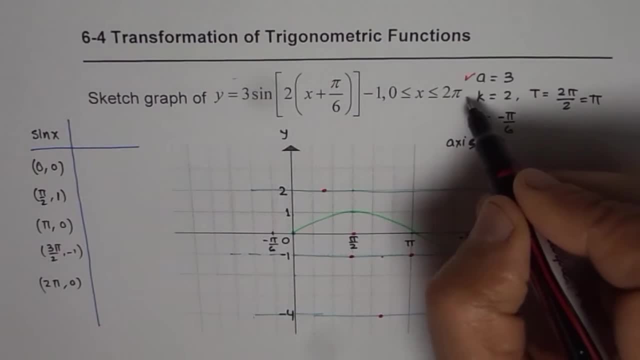 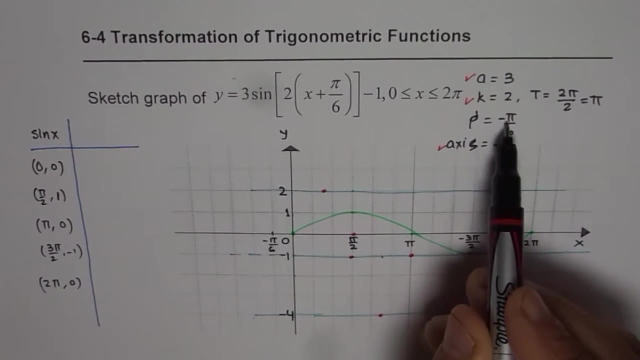 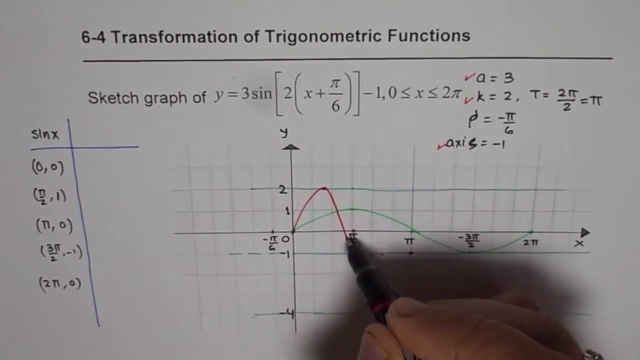 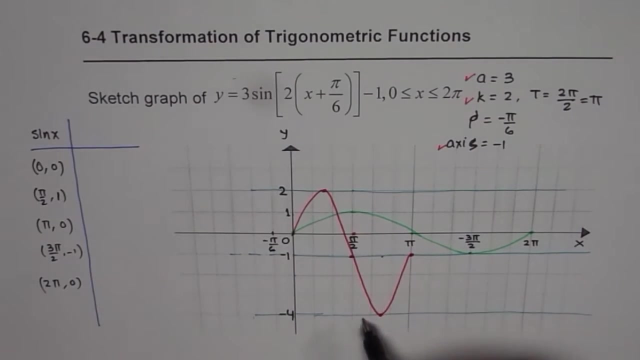 all transformations. We have incorporated these 3 and now we will draw our sine wave and we will incorporate that at the end, right? So what we have here is 1 wave which is kind of like this: Do you see that? So this is 1 wave we have where we have not incorporated minus pi by 6. But we have. 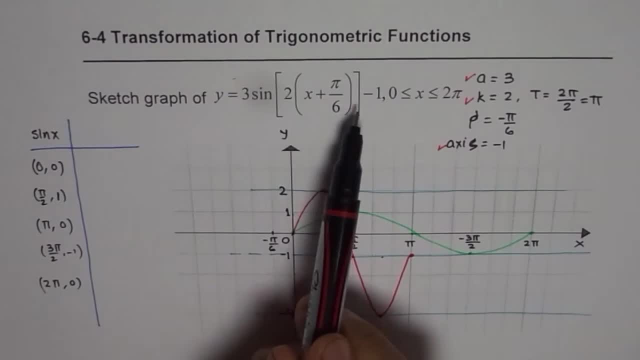 incorporated vertical stretch, horizontal compression and translation. 1 unit down Now, finally, finally, we will incorporate translation also. So when you do translation by pi by 6, then 1 unit is pi by 6.. All these points get to the left by 1 unit. 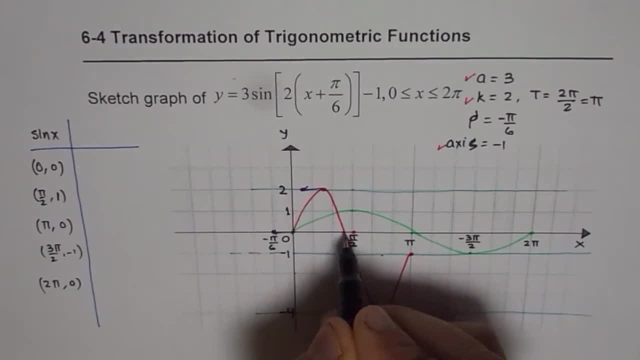 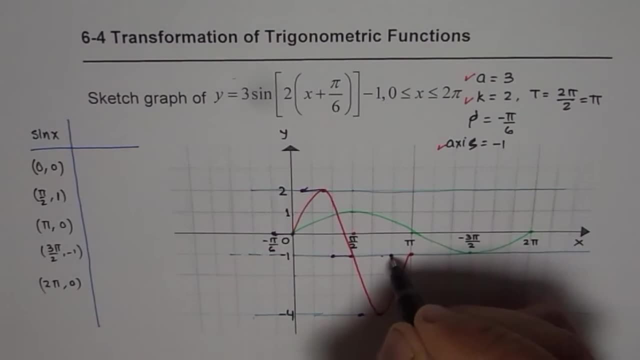 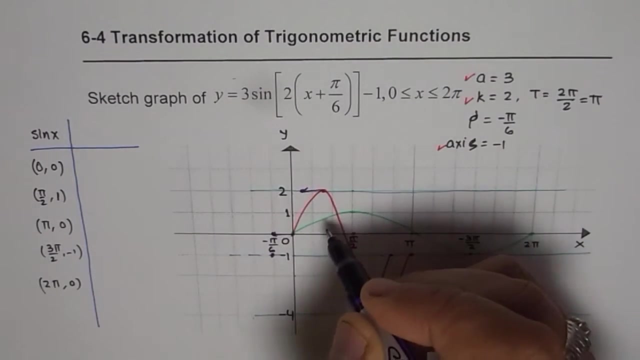 So this comes here. Do you see that? So I will translate all these points 1 unit to left, And then again draw my wave. Oh sorry, this should be here. So this is wrong. This should have started from here. 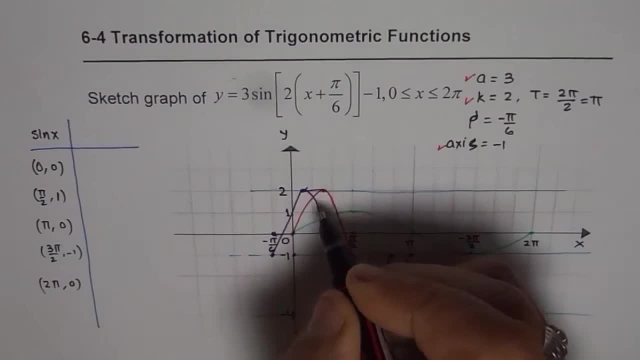 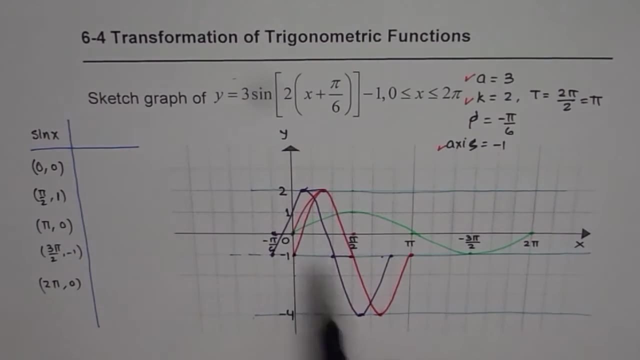 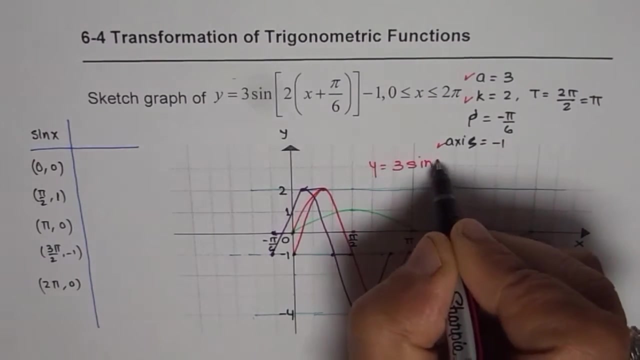 So that is how my wave will be. So let me make this correction, Sorry for the mistake that I should have started because we translated down also right? So this was our wave. So red 1 represents the wave. y equals to 3 sine 2x minus 1.. So that is the red wave, Since we have two waves. 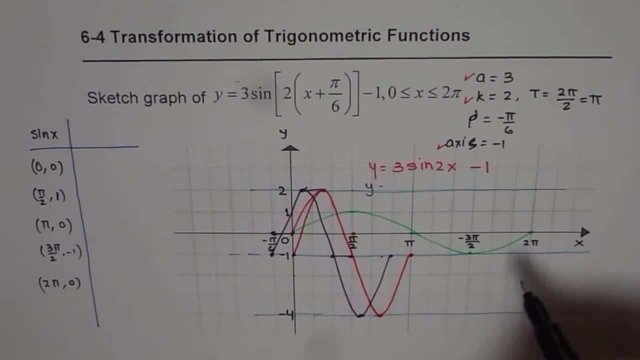 into pi. we'll repeat this wave and then draw the next wave so that we get two waves within the given time period of 0 to 2pi. okay, So we have one wave here. So if I repeat it I get maximum after. 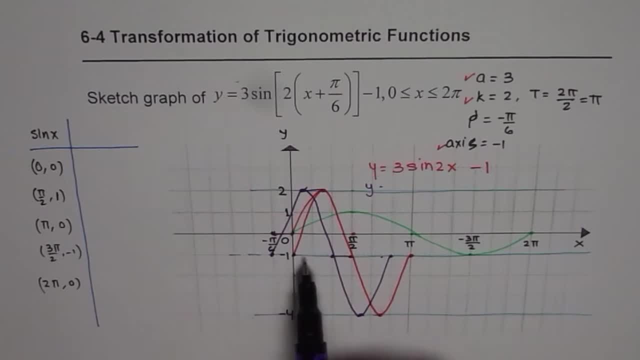 1 and a half of this unit, right? So we are not talking about pi by 6 and pi by 12 at present, but we're just counting the graph units, right? So what we have is maximum at 1 and a half of this. 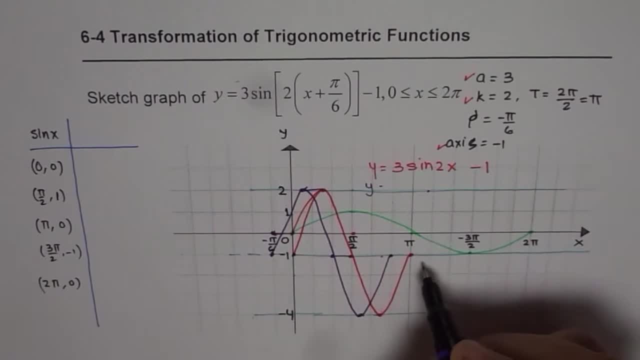 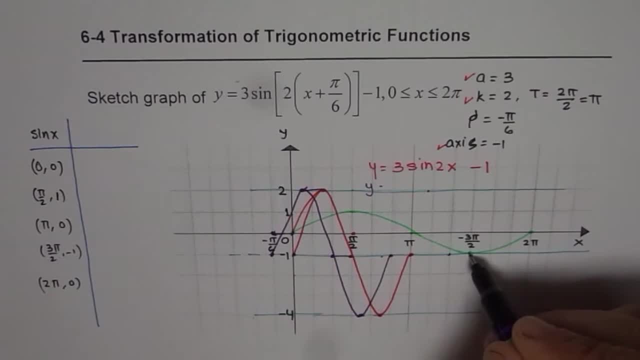 1 and a half. we get the values, which is 3 from here, 1,, 2,, 3, right, And 1 and a half from here, which is right there, and then the 0 at pi by 6 less. 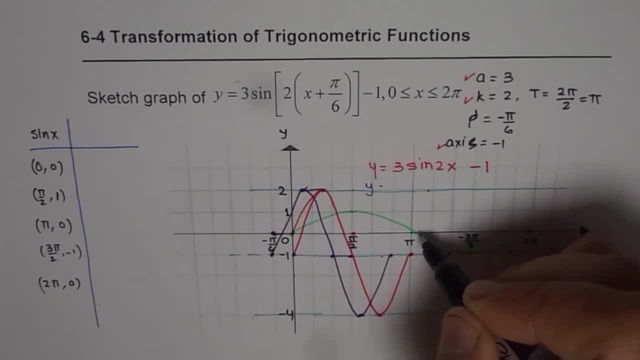 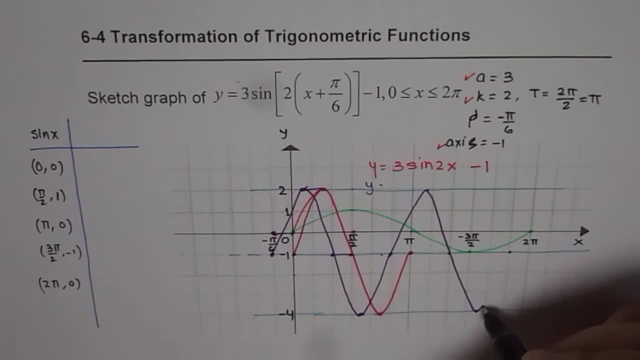 So we can complete these waves and draw the second wave correct. So that is how you can draw the transformed function, using translations, compressions and stretches, as I have shown you. But the idea here is that you can actually combine vertical and horizontal stretches. 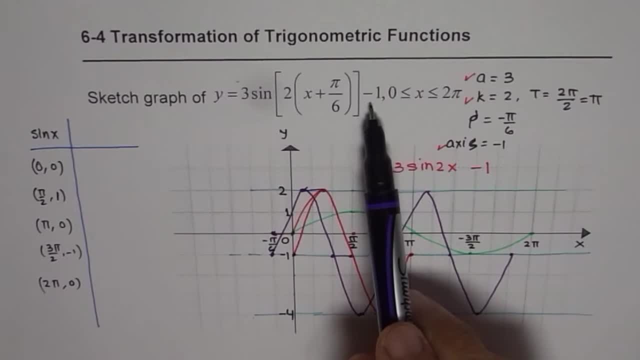 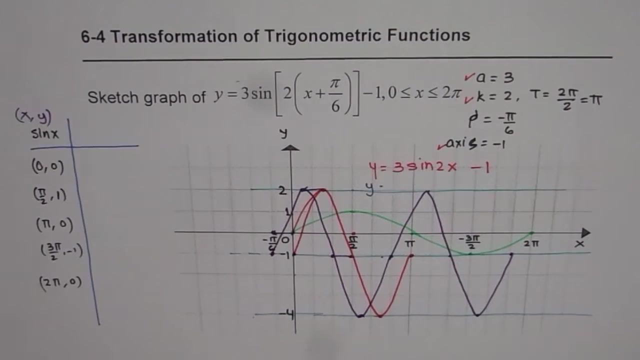 and compressions and the vertical translation in one shot, Then do the horizontal translation and after that repeat your wave. So that is one way of doing it And of course, the other way is we can use the image points. Now, as you can understand, transformation of a coordinate point: x and y on sine of x. 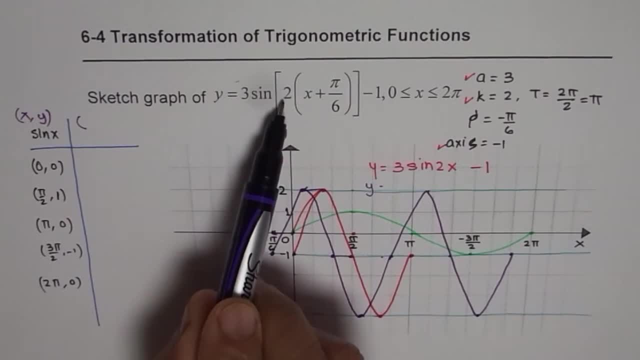 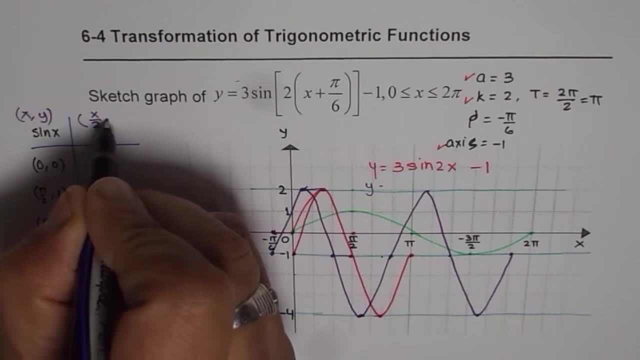 will be kind of: x points will be half and minus pi by 6.. So x points will be x divided by 2 minus pi by 6.. That is the image of the x coordinate points. y coordinates will be minus pi by 6.. 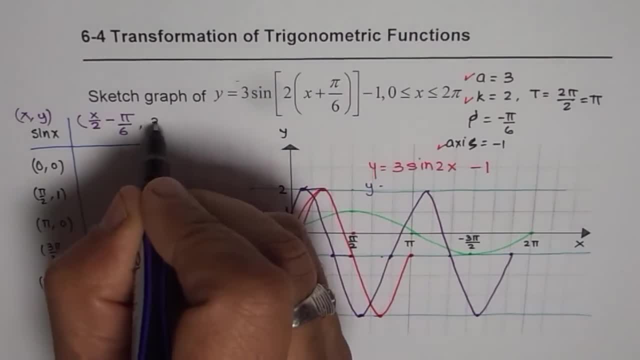 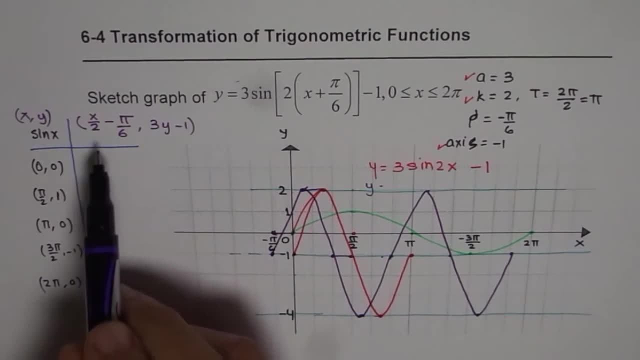 y coordinates will be 3 times minus 1.. So 3 times y point minus 1.. So that becomes the change in y right. Now, applying this transformation, we can get transformed points directly from the key values, and that is a very effective way of getting to the final transformed function right. 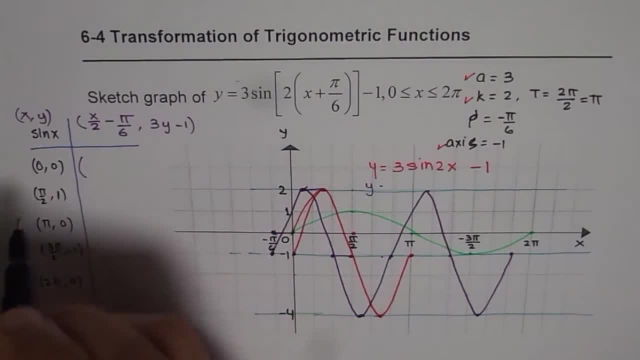 So let us do these calculations. So for the first point, we get 0 divided by 2. Minus pi by 6. That is the x value. The y value will be 3 times 0 minus 1.. Do you see that? 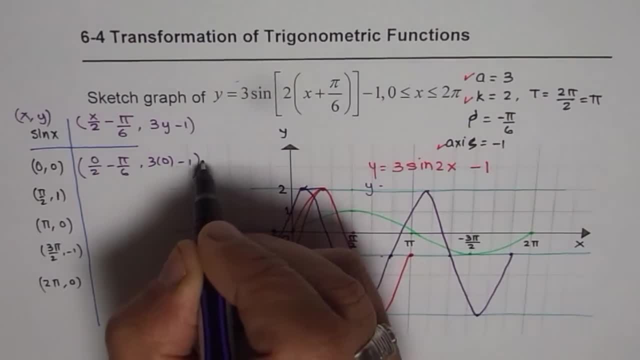 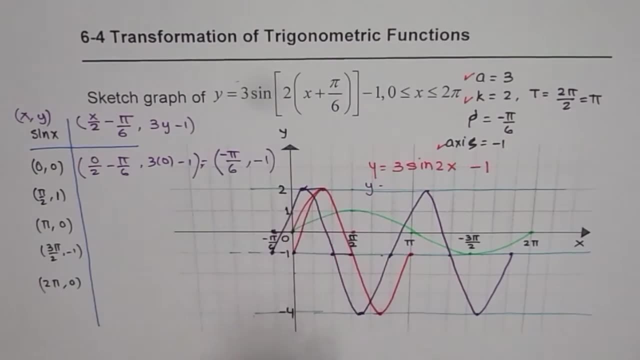 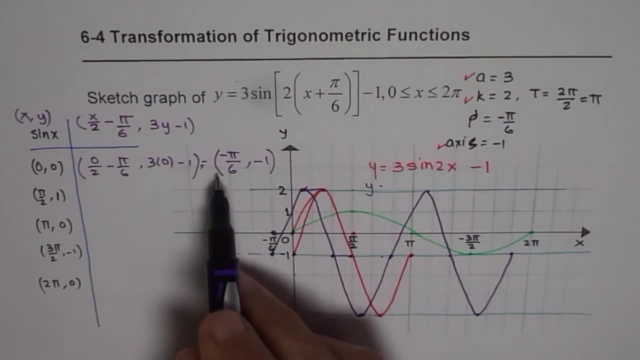 So when you solve this, you get minus pi by 6.. So that is the same as minus pi by 6 and the y value is minus 1, right? So basically, what you see here is the starting point: Minus pi by 6, minus 1.. 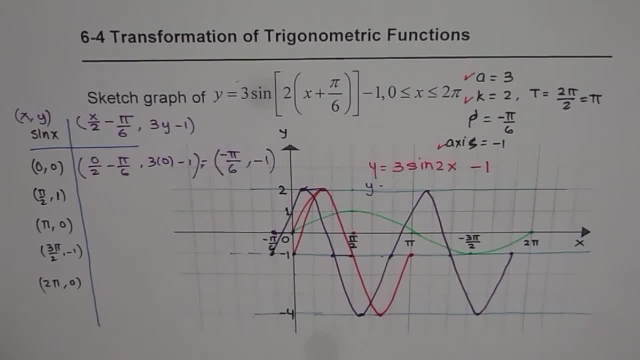 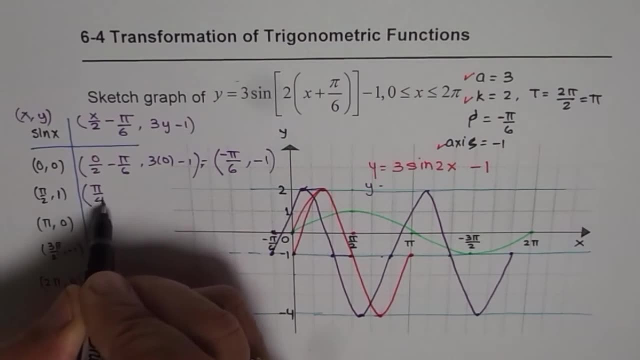 Do you see that It matches with your graph? Perfect. Now the other point. next point will be half of this, which is pi by 2, half is pi by 4.. Minus pi by 6. That is the x coordinate. 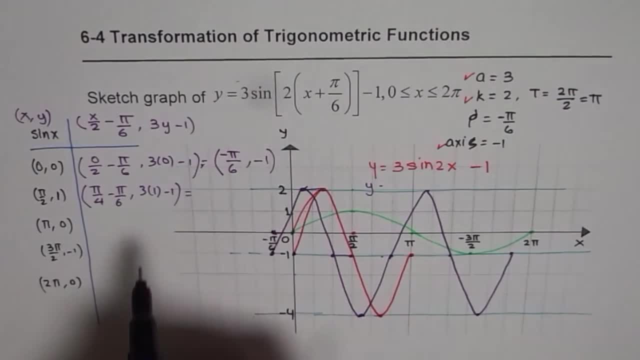 And y will be 3 times 1 minus 1, right, So here the common denominator is 12, so we multiply this by 3, this by 2, 3 minus 2 is 1.. So you get 1 pi by 12.. 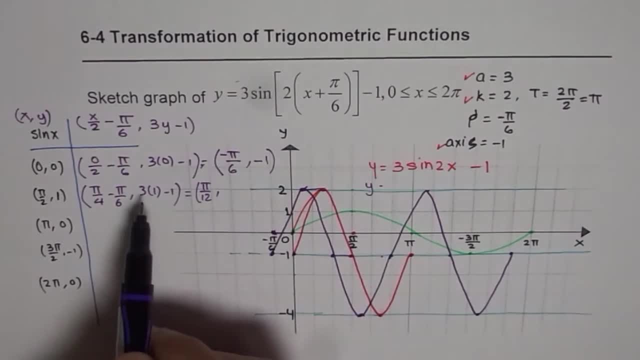 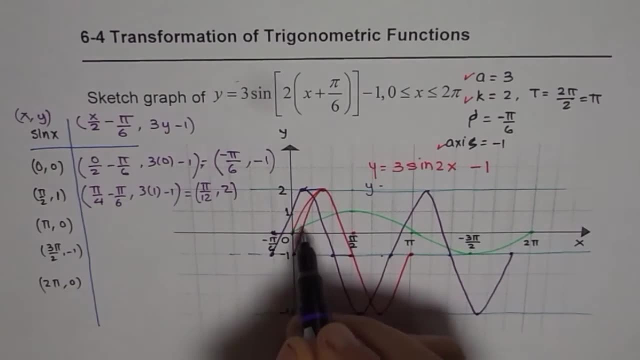 So you get pi by 12.. And the y value will be 3 by 12.. 3 minus 1,, which is 2, right? So there you see. each division was pi by 6.. So this is pi by 12, half of pi by 6.. 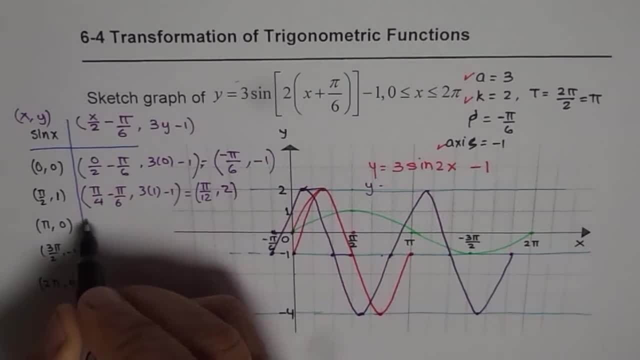 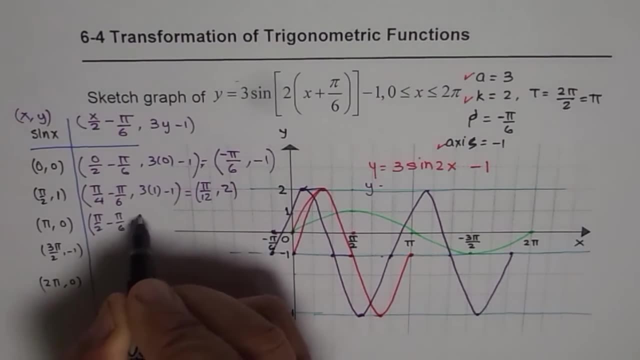 And the y value is 2.. Do you see it matches. So likewise you can do this calculation: Half of pi by 2 minus pi by 6, 3 times 0 minus 1, correct? So here the common denominator is 6 for you. 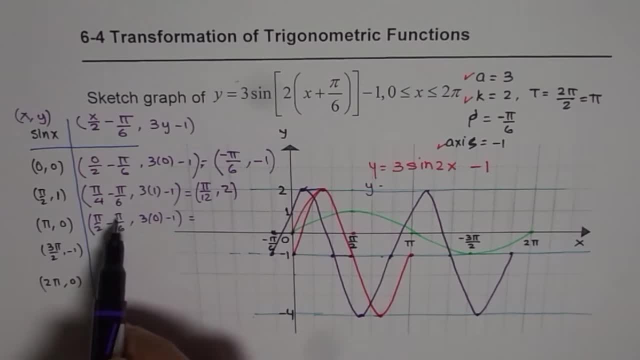 So you multiply this by 3.. 3 minus 1 is 2.. 2 over 6 is 1 over 3.. So you do all that calculations, you get pi over 3, and the value here will be 0 minus. 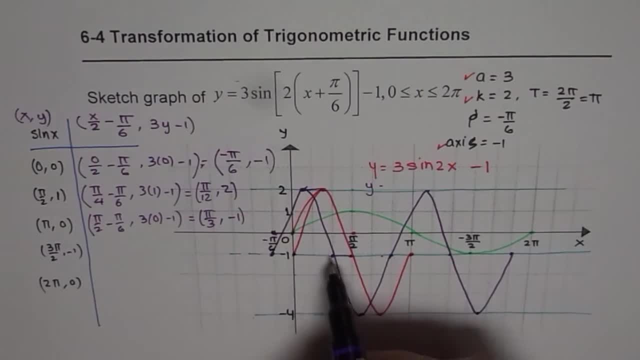 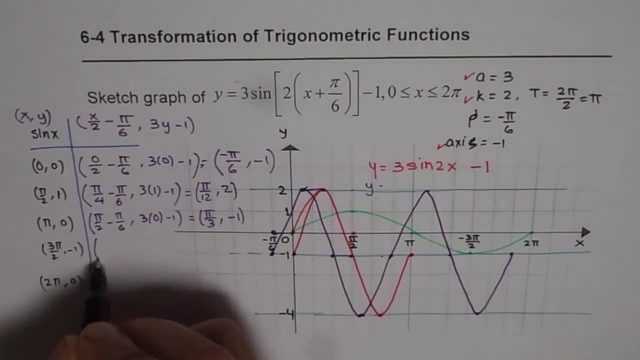 1 as minus 1.. So you get a minimum- I mean a minus 1, at pi over 3, which is 2 pi by 6, correct? Then next point will be 3 pi by 2, half of this is 3 pi by 4.. 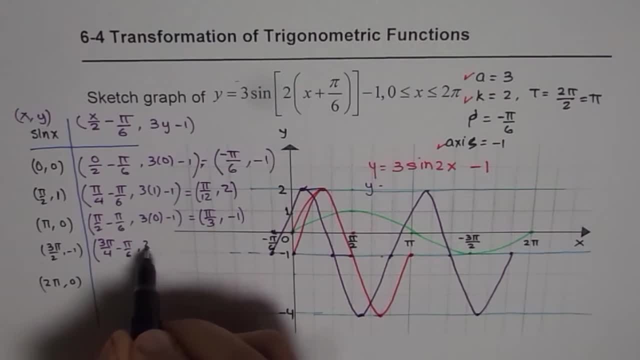 Minus pi by 6.. The y value will be 3 times minus 1 minus 1,. correct Here the common denominator is 12.. To get 12, you'll multiply this by 3, so this becomes 9, this by 2.. 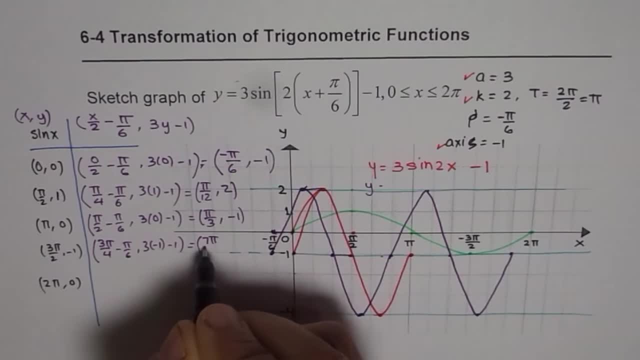 So you get 9 minus 2 is 7,, right. So you get 7 pi by 12, and the y value will be minus 3 minus 1, which is minus 4.. And that gives you absolute minimum for this at 7 pi by 12 minus 4.. 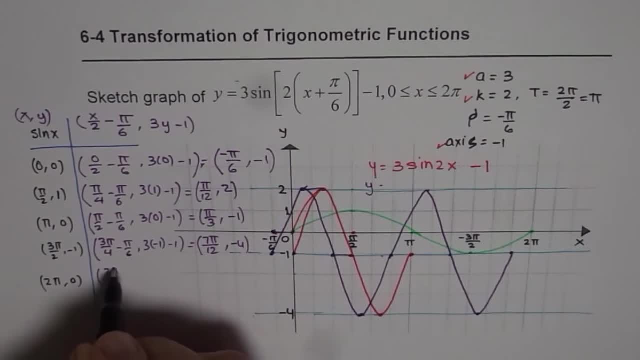 Do you see that The last point is half of 2 pi minus pi by 6, and the y value will be 3 times 0 minus 1.. So that is pi minus pi by 6, or you can say 6 pi by 6 minus pi by 6, or 5 pi by 6.. 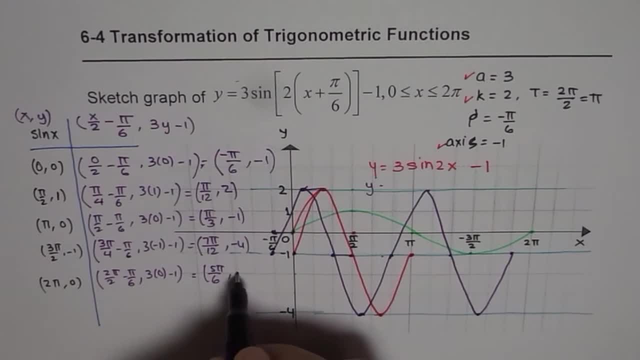 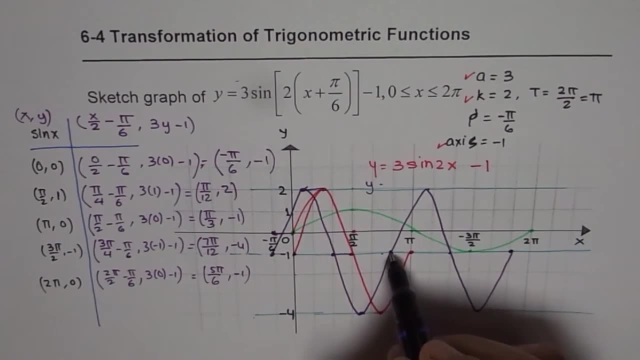 And 3 minus 1, 0, 3 times 0 is 0, 0 minus 1 gives you minus 1.. So that's the last point for us. 5 pi by 6, I mean here The last point for us, right? 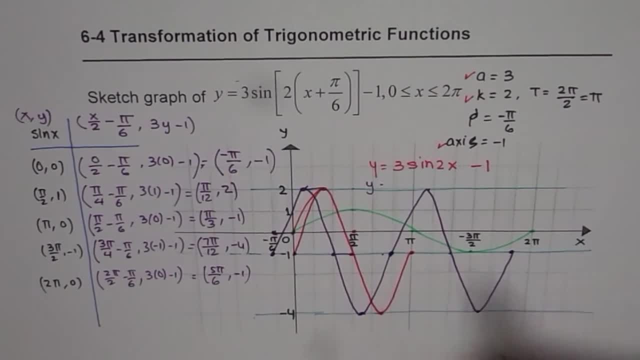 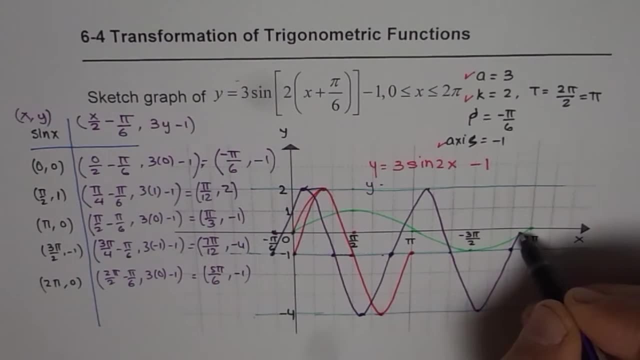 So you get one full wave here. you get the point Now within 2 pi you have to extend. So you just extend this, draw a line symmetrical, and so 1 and a half it is kind of going there. 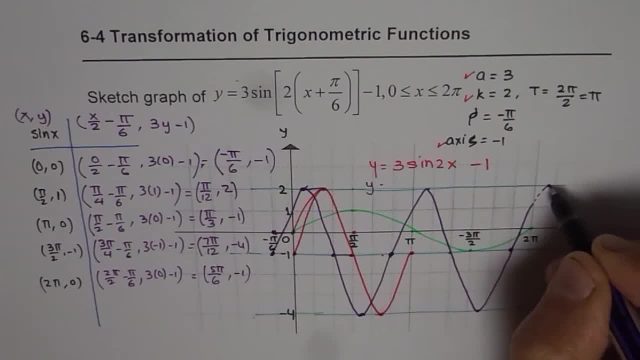 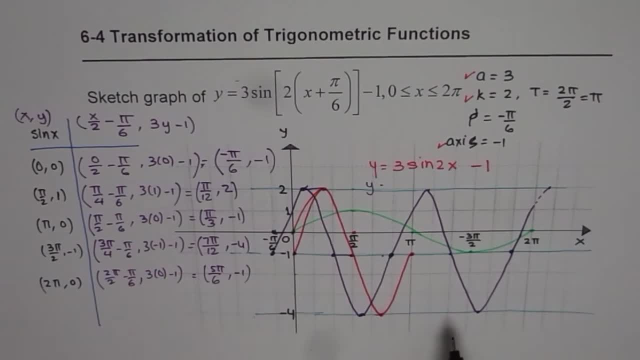 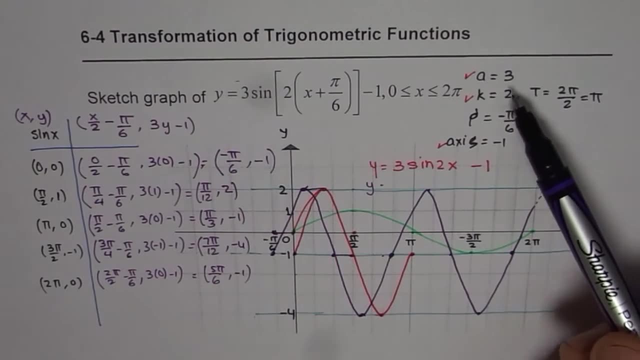 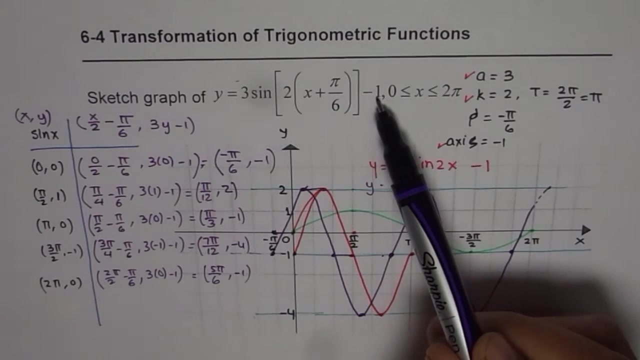 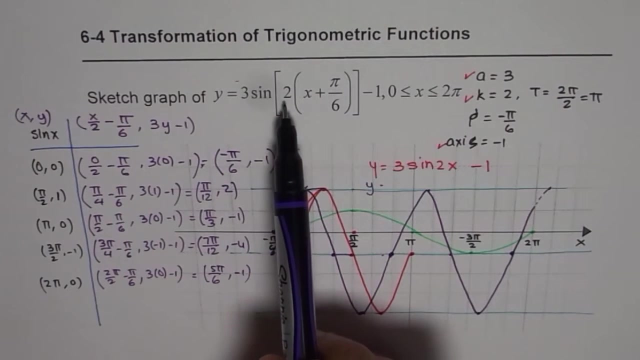 a transformed function. So what you learned here is that if you are given a transformed function, we can analyze change in amplitude. the phase shift time period axis- Axis is minus 1- translates pi by 6 to left: time period becomes half of 2 pi. that is pi and the amplitude becomes. 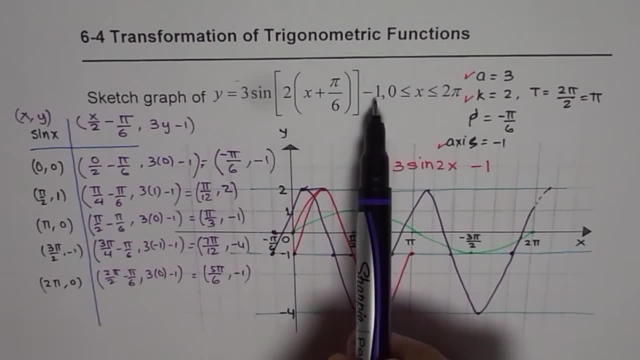 3. Now that amplitude and the axis changes the range right, The range now is from minus 4 to 2 and within the domain of 0 to 2 pi. this time you are going to have two waves, since k is 2,. 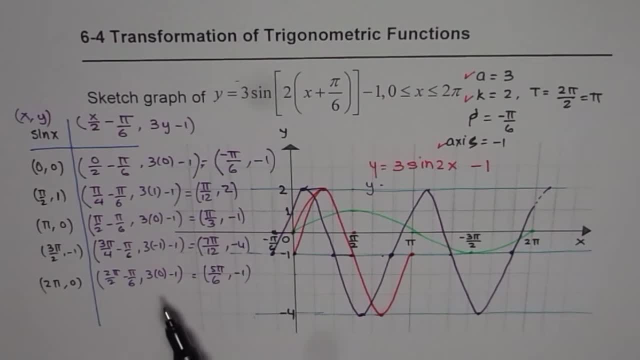 correct. And now you also understand the second method of plotting the points and then getting your equation. So, if you go with the five key values for sine x, which are at 0 maximum, so this was our key values, five key values started with, and transform them with the help. 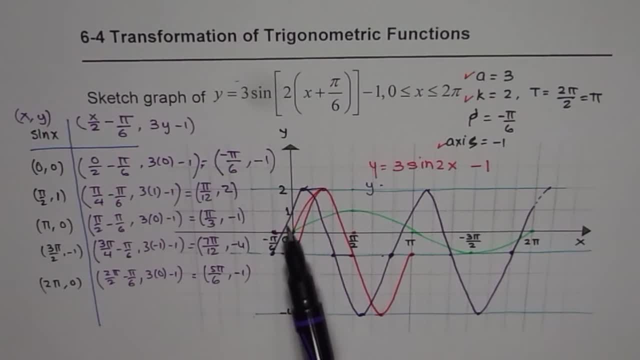 of image points, you get your image points. If you connect those image points, you get your wave. Now, since the interval we're talking about is 0 to 2 pi, you need to repeat this periodic function so that you could sketch it from 0 to 2 pi, correct? So that is how you get a transformed. 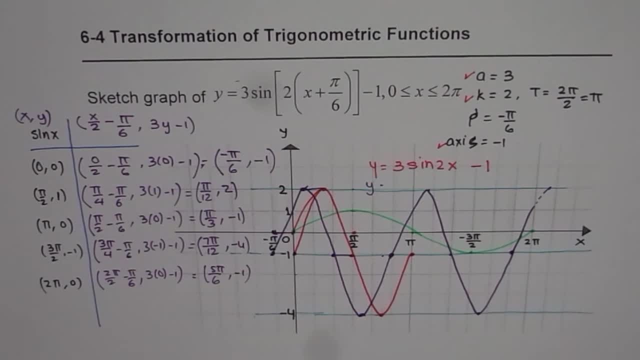 function. I hope it helps you to understand all the concepts of transformation of trigonometric functions. Thank you and all the best.